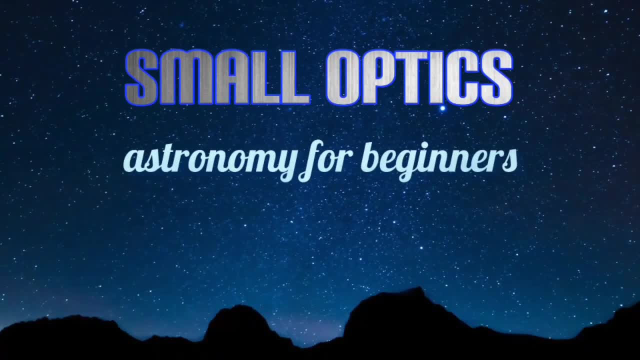 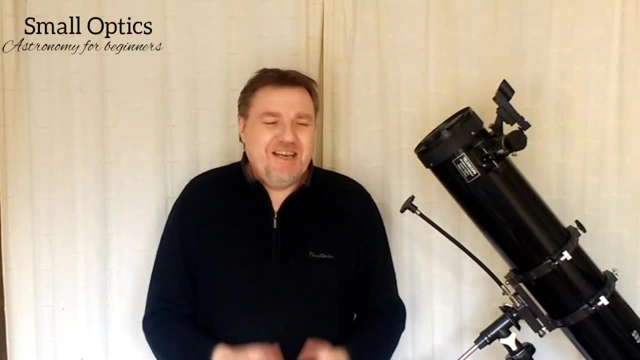 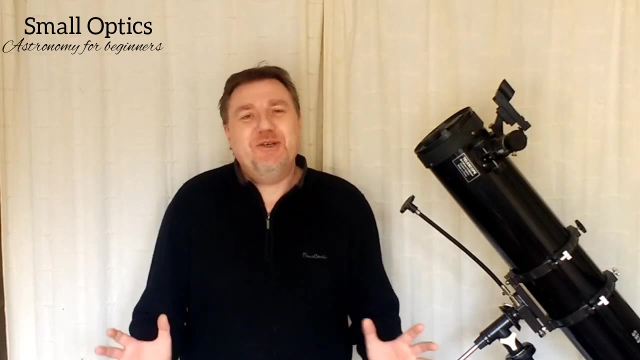 Hello, welcome to my channel, Small Optics. my name is Jason, So you want to get started in the hobby of astronomy? Well, first off, congratulations. you couldn't have chose a better hobby to get involved in. Well, it certainly kept me entertained for the past 30 years- put it that way- and every. 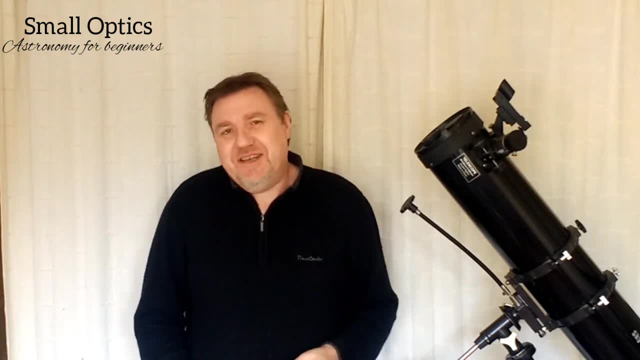 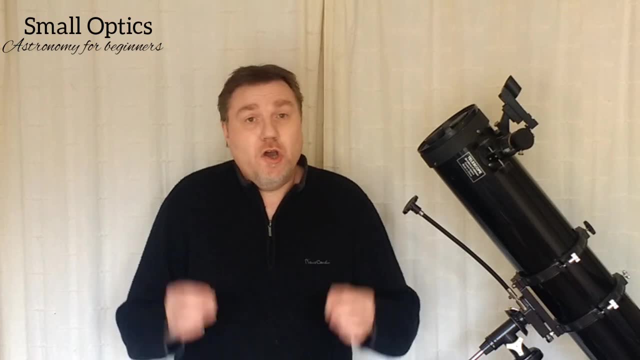 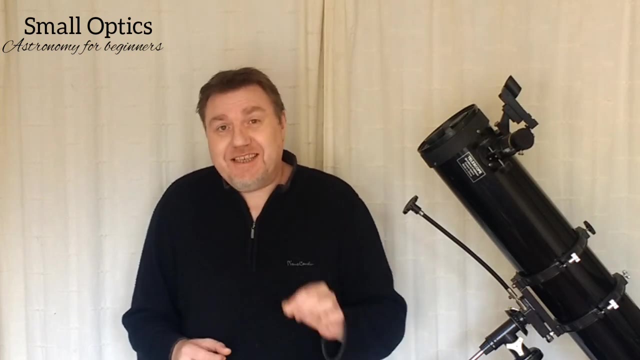 clear night. I go out there. I find new levels of entertainment. Now, the most common question asked when anybody starts astronomy is: do I need a telescope, or what telescope do I need to buy? and the latter is what you should be asking really is: do you actually need a telescope to start? 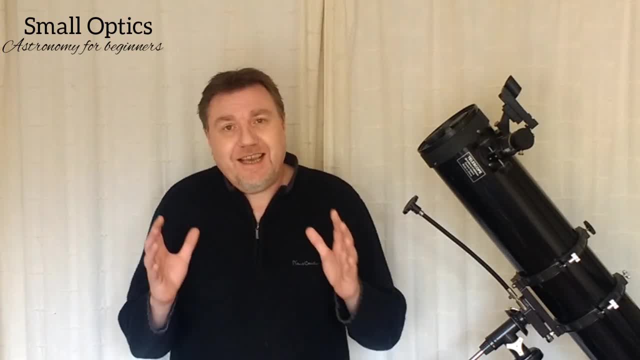 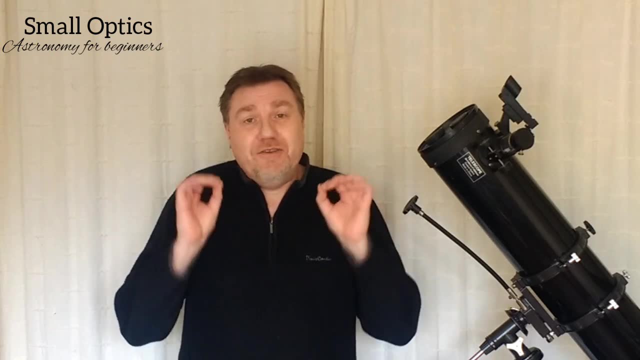 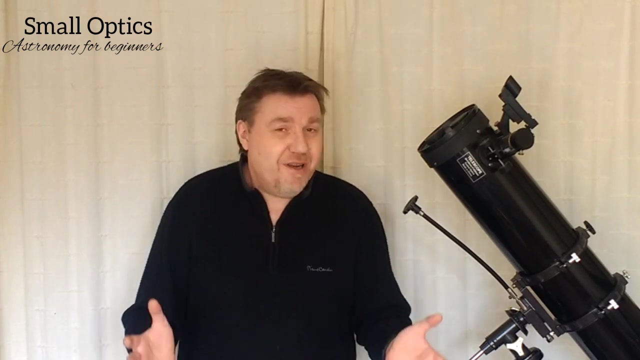 the hobby of astronomy and the answer is a big fat. no, you don't. you really don't. in fact, I'd encourage you not to buy a telescope for at least nine months or something like that. I've actually been into the hobby. I know you're not going to like it's just irresistible. there's. 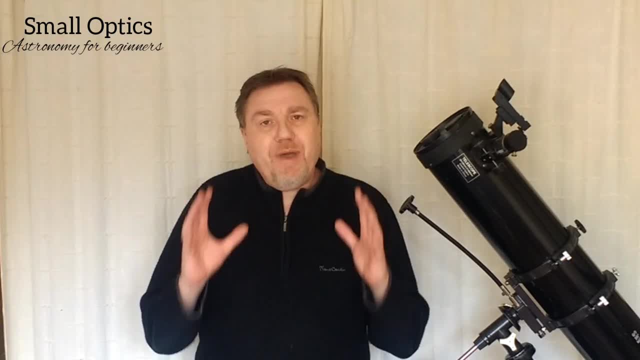 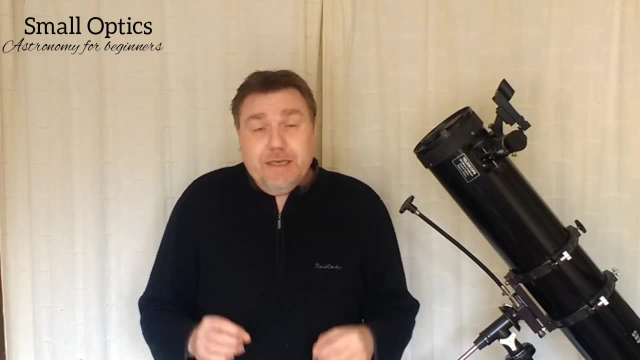 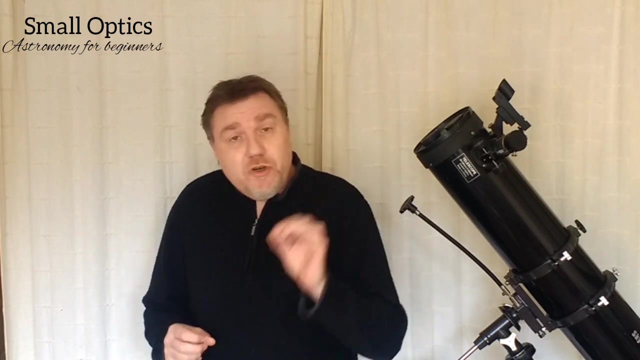 that many, uh nice telescopes out there. Now the best thing to do before thinking about buying any optical aid is to learn your way around the night sky. Now this may sound like it's well. that's a that's a real hard task. you know, how am I supposed to learn my way around all that? but once you. 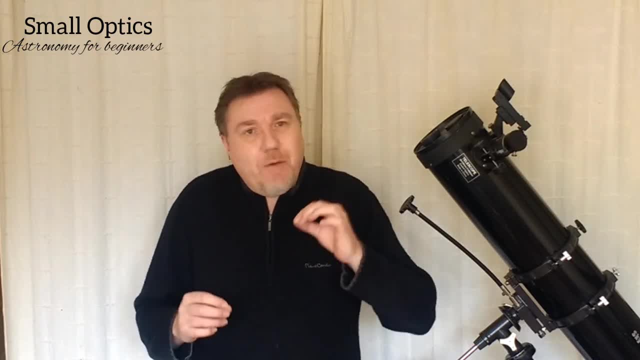 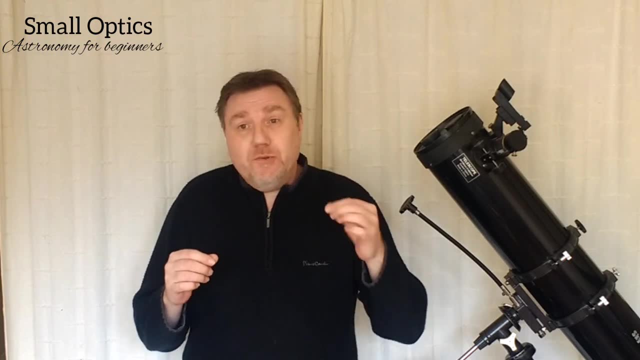 actually get started with astronomy, you're going to be able to learn your way around the night sky. when you get started, you'll find just how how easy it becomes. and I mean, I haven't got no super memory. in fact I've got quite a poor memory, um, but you, I, if there isn't a star up there, really, 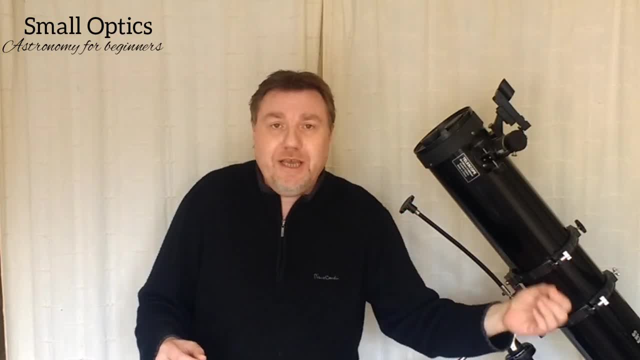 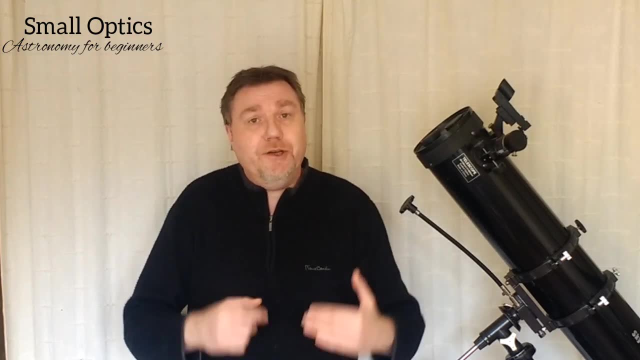 that somebody could point to and I wouldn't be able to tell them what constellation it's in. not because I'm some professor of astronomy or anything like that. it's just that that's the first thing I studied when I got into astronomy. excuse me, and the thing is with learning the constellations. 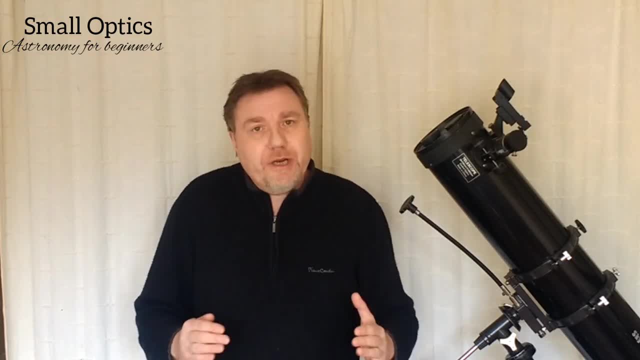 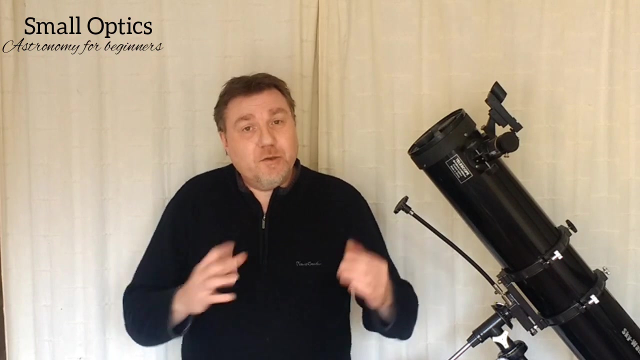 or learning your way around the night sky. you will be using it throughout the time you are into this hobby. basically, I mean you constantly use the constellations. they're going to point you on to bigger and better things. now, what I mean by lead you on to bigger and better things is you use 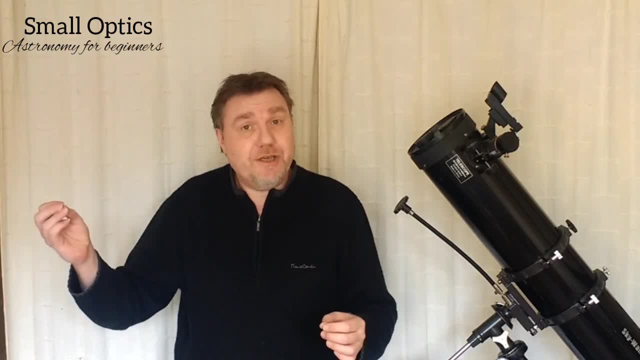 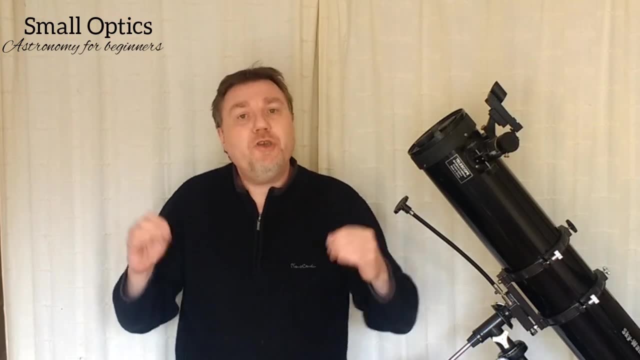 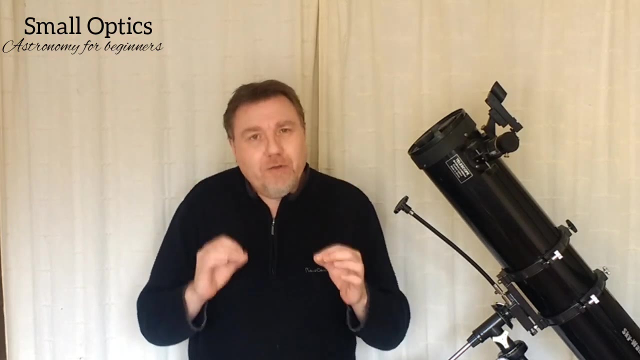 constellations to point to a lot more interesting targets that are up there: some of the deep sky objects, some of the galaxies and the star clusters. so all the time you'll be using the constellations, constellations, constellations. so, um, you know, it's a real good thing to start off learning them from. 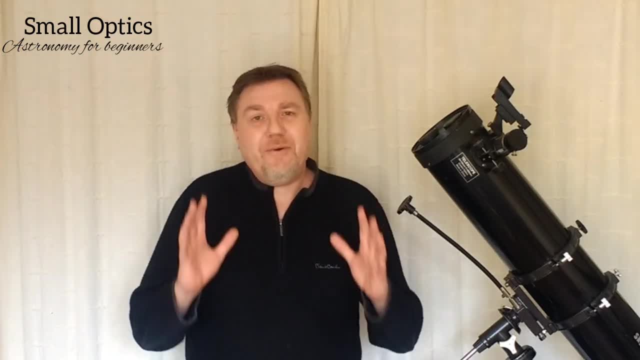 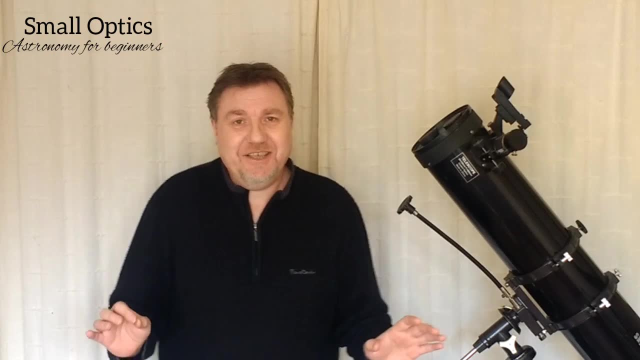 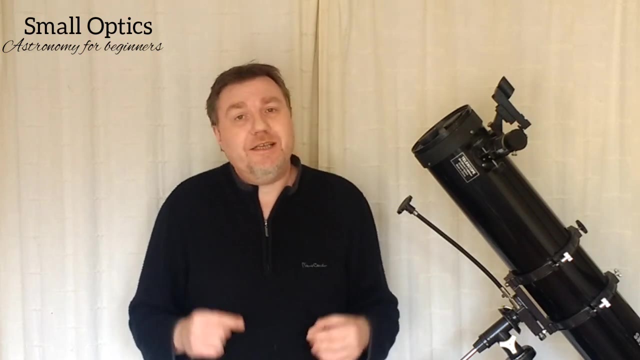 really early in the in the hobby. now, in total there are 88 constellations and I don't mean go out there and learn 88 constellations in a week, um. a- that's just going to totally overwhelm you, and b- you'll not be able to do it because it'll actually take you 12 months to learn all. 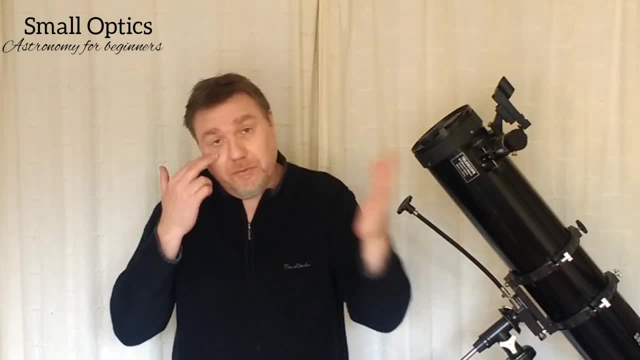 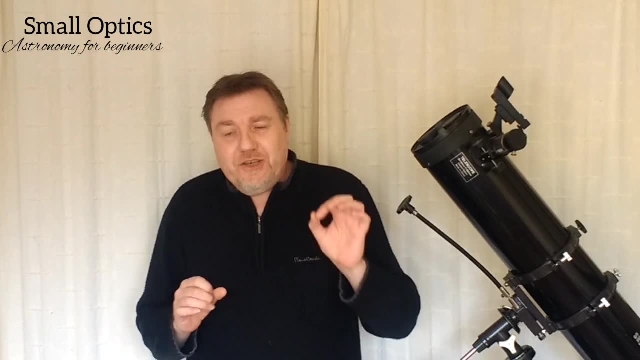 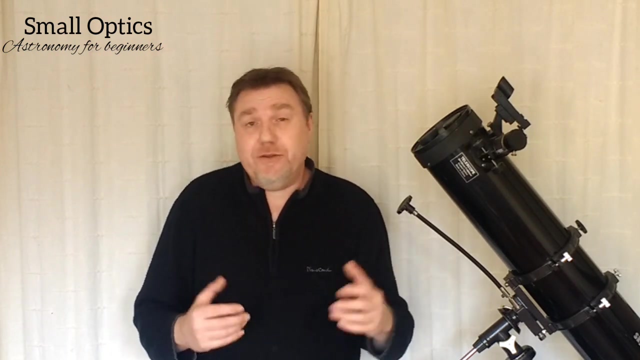 the constellations, constellations, because it takes 12 months for them all to complete the cycle around the axis, okay, or should I say around the pole star. now you don't have to learn all 88, no matter what, because we can't see all 88 constellations, and that all depends on whether you live on the north or 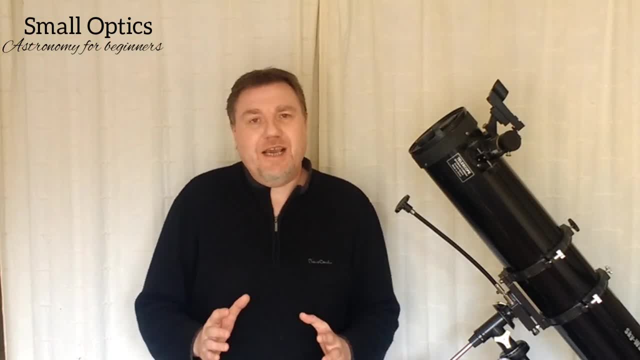 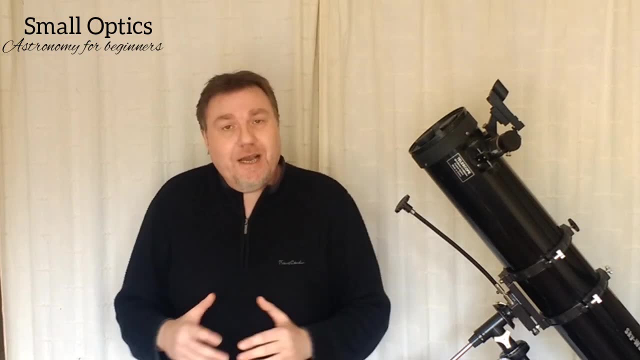 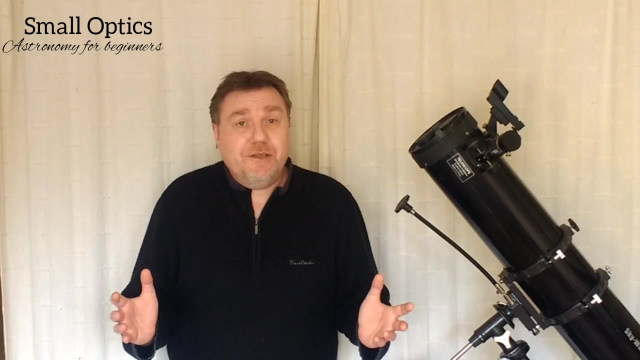 southern hemisphere. now, when it comes to learning the night sky or the constellations, um, I can't stress more than buying a good book, and I do say book rather than app. okay, the thing is with books, and it's not because I'm old-fashioned or anything like that, um, you just absorb information better. you can go through a book at. 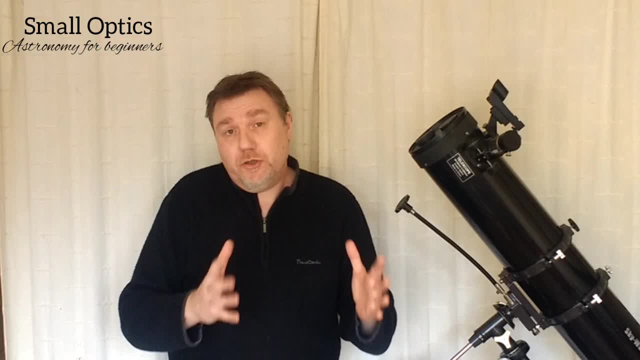 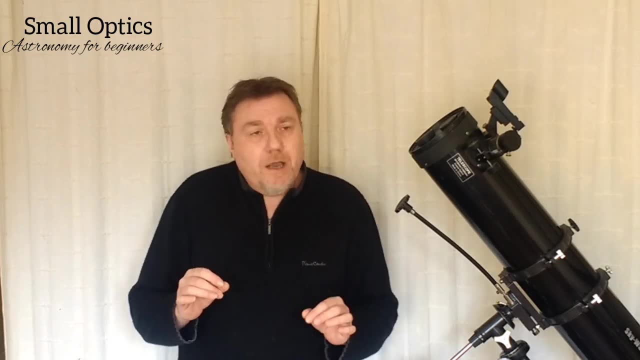 your own time. you'll learn a lot more from a good star chart than you would watching a hundred videos. okay, now the books to go for. um, I mean, I could. I could recommend. there's hundreds out there that are worth buying. okay, but without sounding patronizing- and I don't mean to sound this- 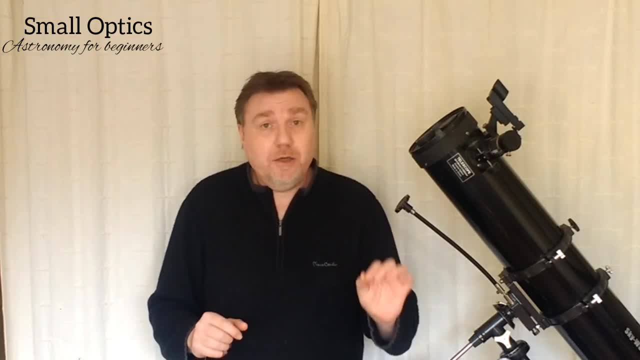 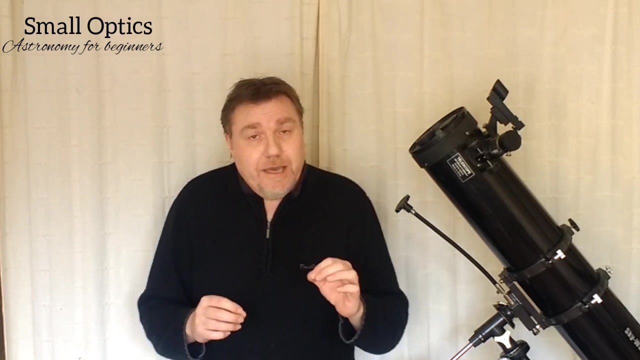 patronizing at all. okay, no matter how old you are, whether you're 16 or 60, go for. if you're a total novice, okay. and you- you don't know, your leo from your gemini? okay, get books that are aimed at kids, okay. now the thing is with those books. they are still accurate, all right, and they're going to. 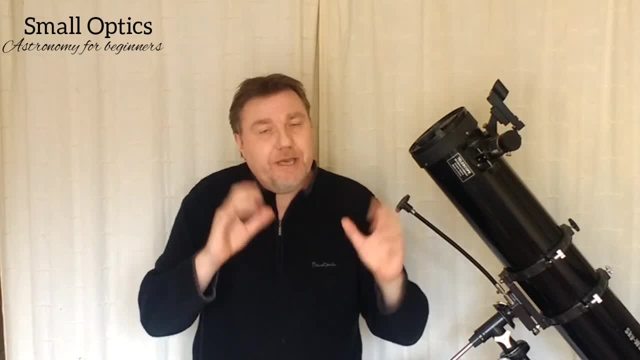 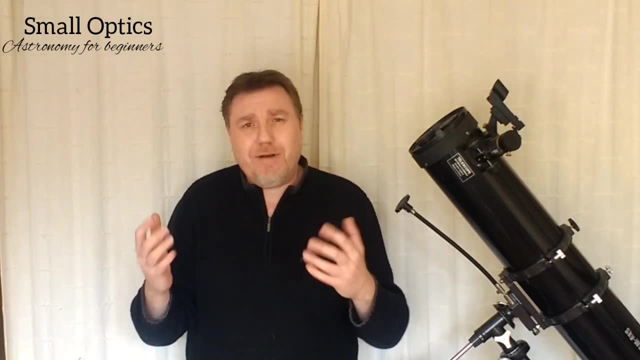 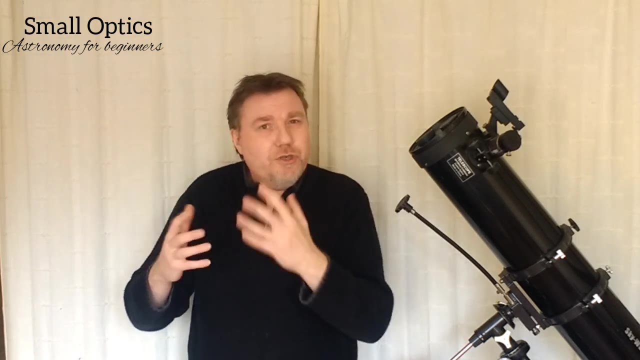 point you in the right direction. but the very basic, the colorful, that easily laid out and the cut out all the jargon, unlike a complicated star atlas where there's a lot of things on there that are too much at the time. uh, they kind of you know they're going to confuse you, there's going to be too much to take in. 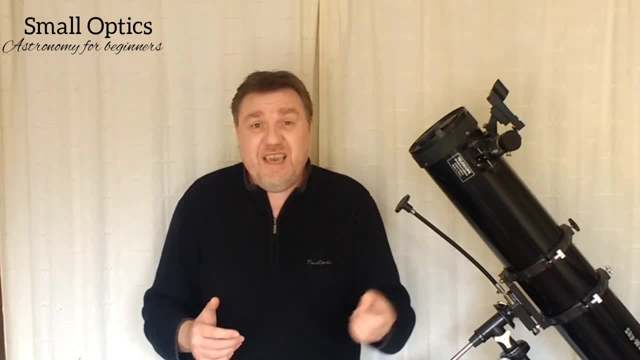 where these kids books like astronomies- uh, for for beginners, or you know that are aimed around about the 10 to 12 um age group- are brilliant for learning when you're first starting out. so don't be put off by the books that are aimed at kids. 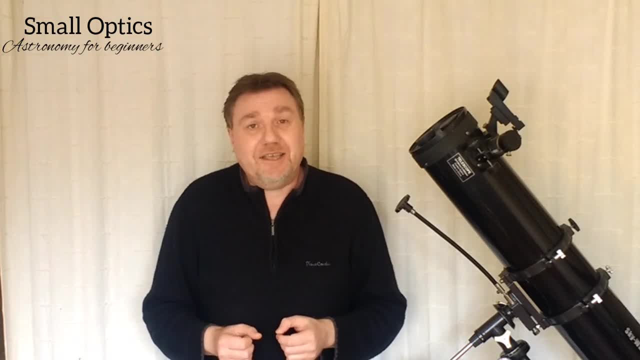 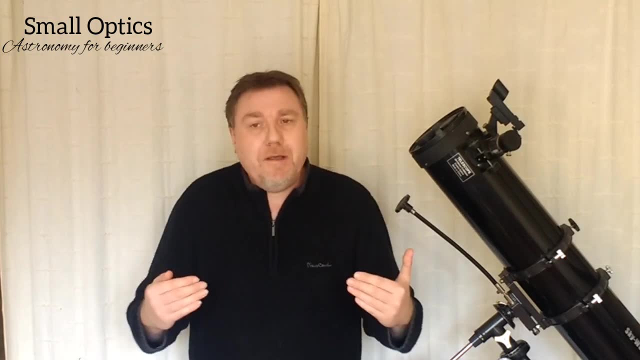 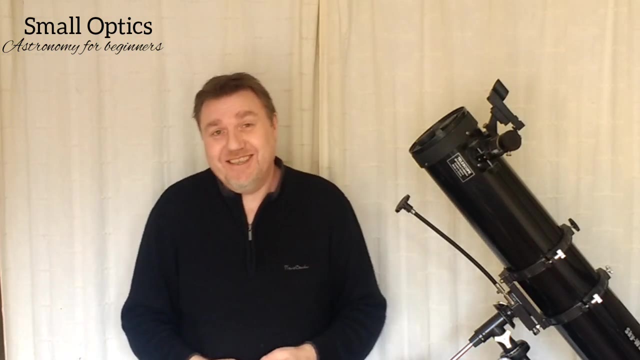 you know, don't think- well, this is a bit babyish- like they really will help you and it's a massive step into um being. you'll quickly go from being a beginner to a seasoned astronomer just by learning your constellations. now I briefly uh talked about, uh, some optical aid, telescopes and such like at. 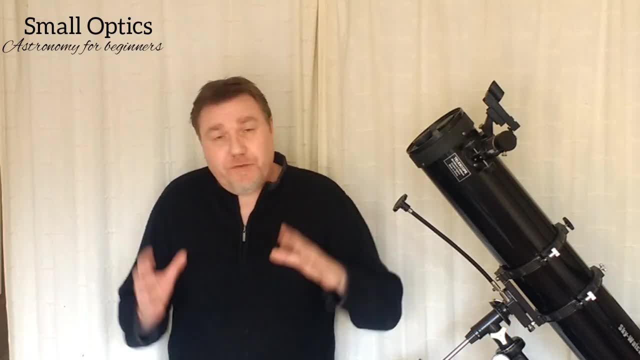 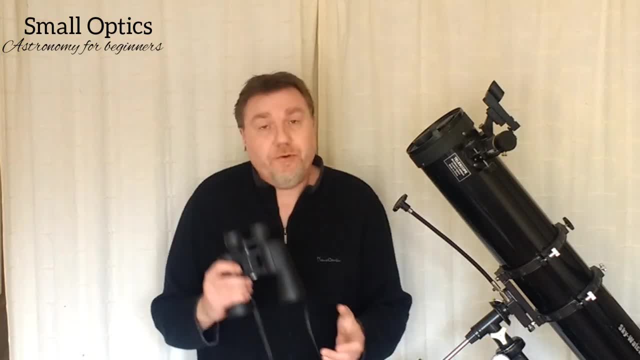 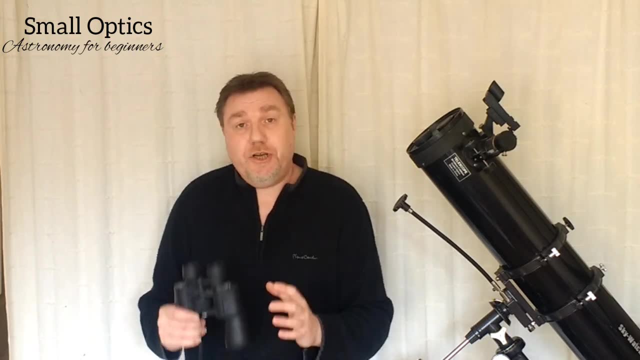 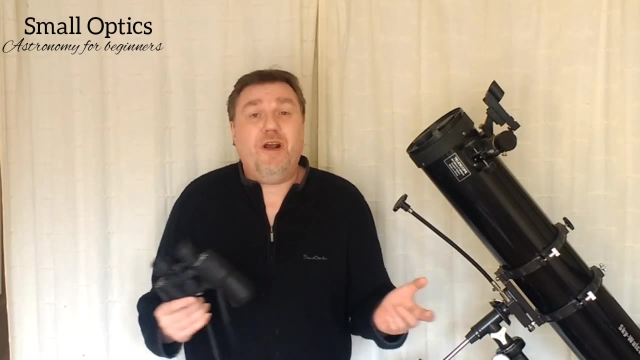 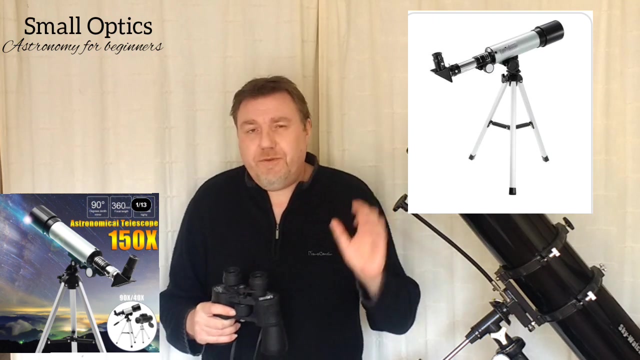 don't overlook or underestimate binoculars for astronomy. okay, a good pair of binoculars is a hundred times better than a cheap department store telescope. okay, in the community they're called trash scopes, basically, or toy scopes. okay, you may have seen them. they have an aperture of around about 50 millimeters, something like that. trust me, you may have好了 igona svenska millones and of course, we wouldn't be able to get this entire thing used. so that's just a basic question, probably the harder one, but yeah, the beauty of with the back, that's your favorite the thing to do and you can get all of your hurdy the way you want. 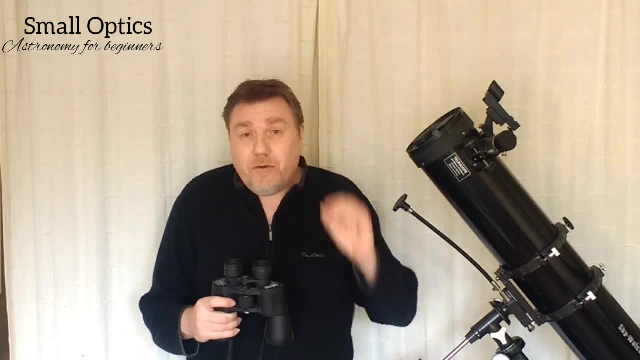 in some have. I've got, uh, black serönacaà. see, you should be very glad to pick up in order to check if the takeoff schedule is good when a fly is going to come. you may as well just get a drinking straw and try looking through that, because that's the sort of 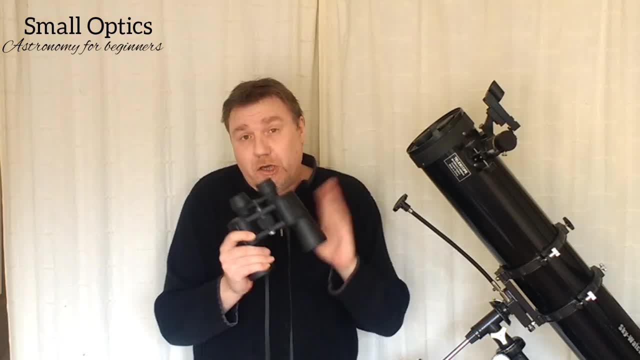 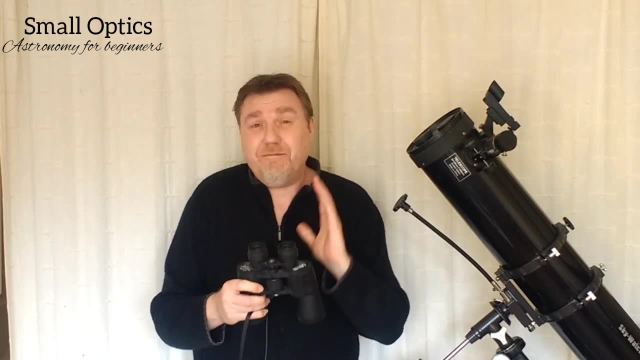 views you're going to regain and, on the other hand, a good pair of binoculars. now they don't even have to be full-size binoculars like this. I mean, these are cheap, budget binoculars and they're absolutely fantastic. in fact, there isn't a clear night where these don't come out with me. I still use them now. 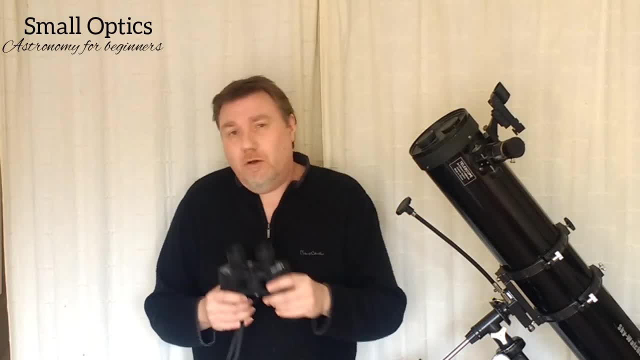 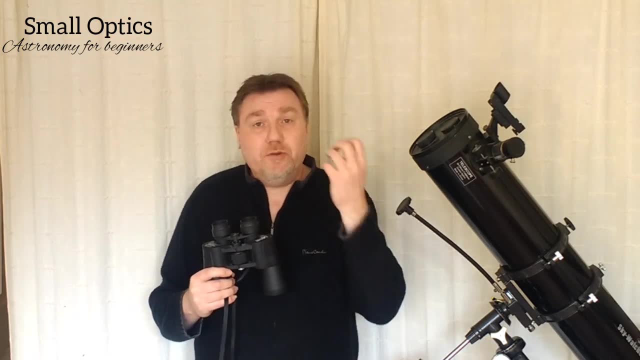 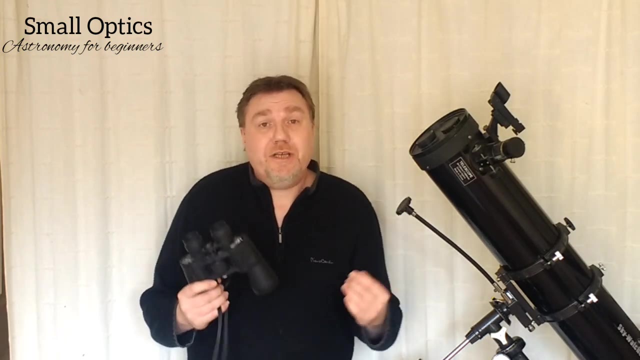 even though I've got a telescope, I still do love looking at the stars through a pair of binoculars. and, like I say, you don't need full-size binoculars like this, just small bird spotting binoculars, walking hiking binoculars, or whatever you want to call them, are fine, just for starting out, I mean. 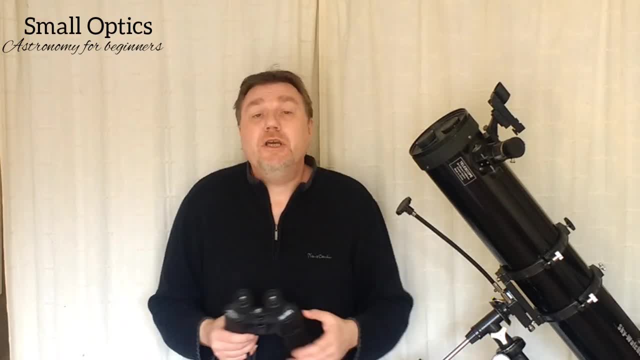 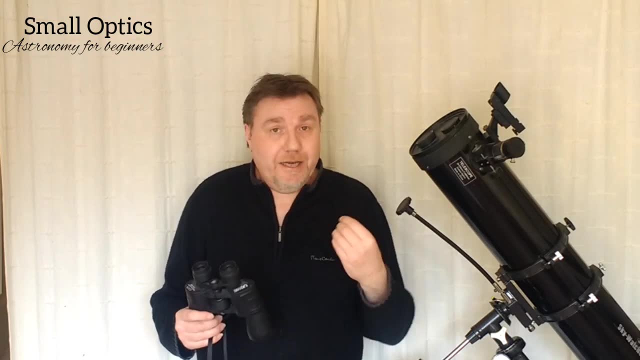 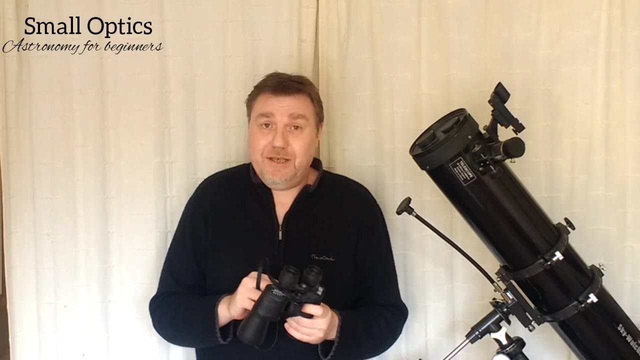 binoculars are going to show you star clusters. they're going to show you the craters on the moon. they're even going to show you some deep sky objects, some of the brighter nebula and galaxies. so if you've got a pair of these or you know, thinking of buying some kind of optical aid. 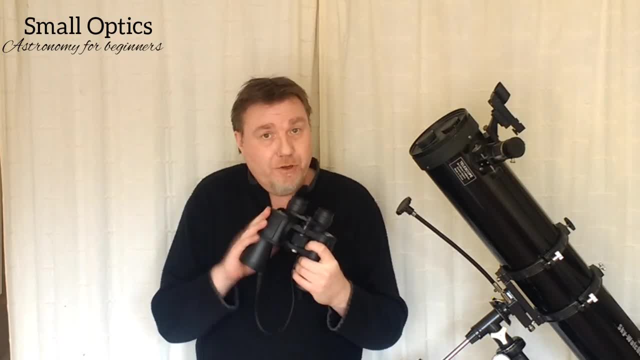 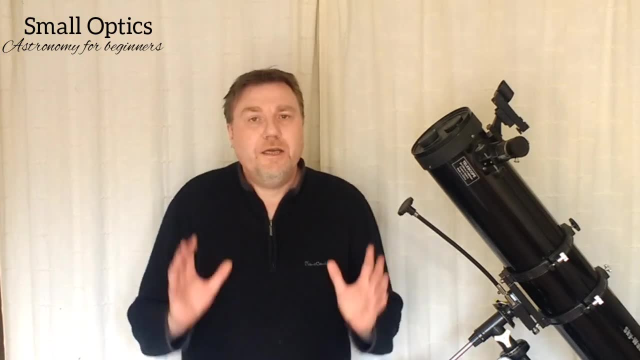 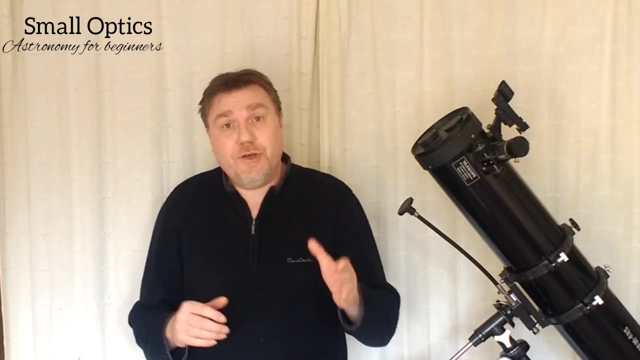 you. you'll be far better off just spending a few pounds on a pair of binoculars before you even think about buying a cheap telescope. Now I will be doing a separate video on choosing your first telescope. so if you haven't subscribed, you know, maybe subscribe and hit the notification bell. 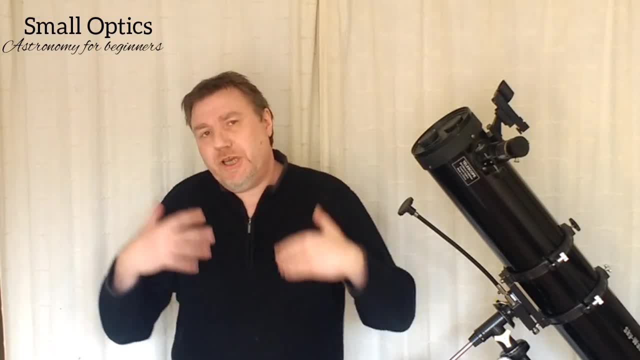 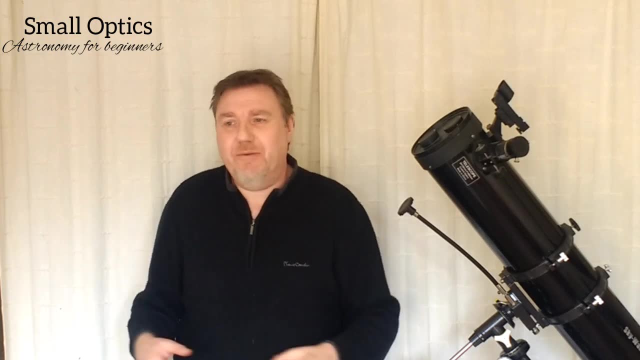 because you don't want to miss that one and I want to keep that one a separate video because there's a lot of things you've got to think about. it's a lot easier than just going out and saying, oh, I'll have that telescope, okay, so stay tuned for that one. Now, probably my top. 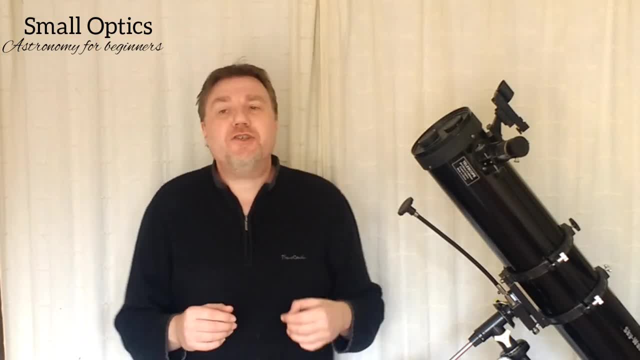 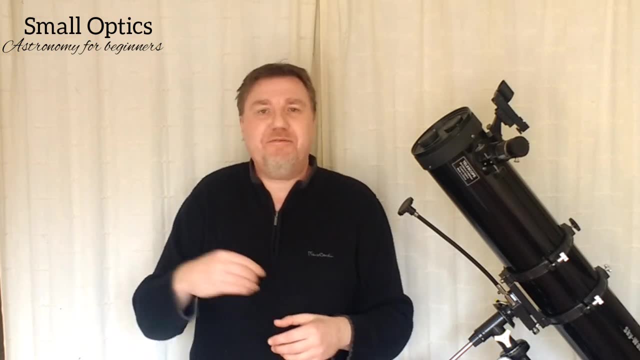 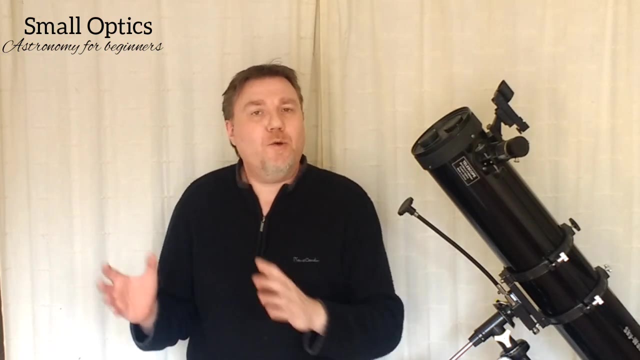 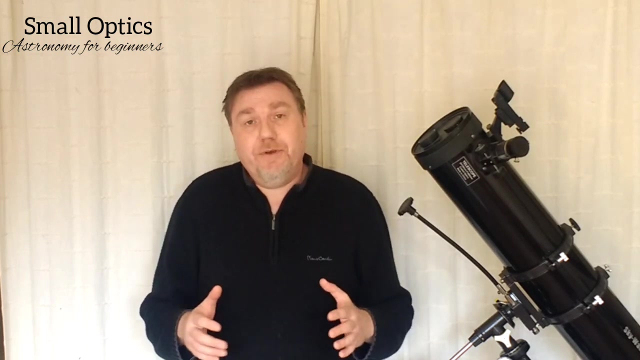 tip for any beginner: something that you're going to learn so much in just a couple of visits, probably a thousand YouTube videos worth, is, if you're lucky enough to have some kind of astronomical club nearby you, I'm joining it. okay, an Astronomical Society Now here in Chesterfield? we're really lucky. 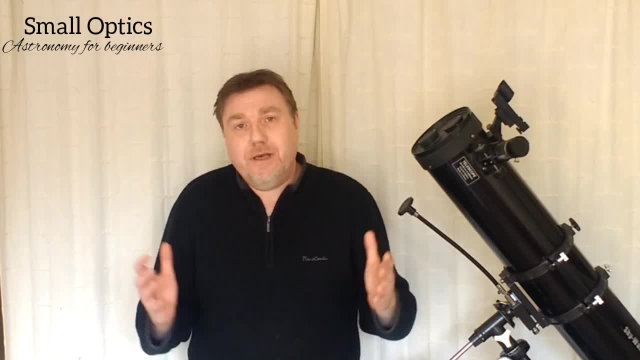 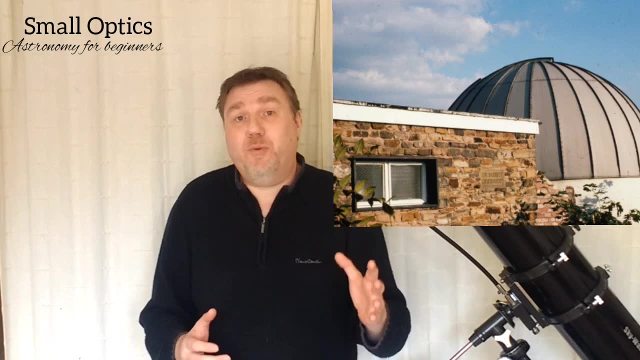 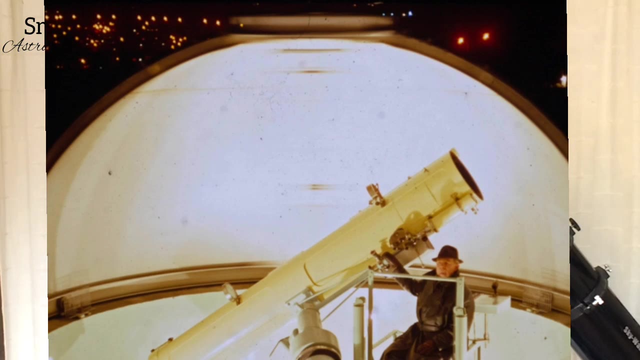 about two miles. that way we have the Chesterfield Astronomical Society, the thing where it all began for me, really. I joined that when I was about 12 years old and I was lucky enough to grow up with a 18 inch Newtonian reflector. and it would be, would be fantastic, was a refractor, a reflector, a Newtonian? 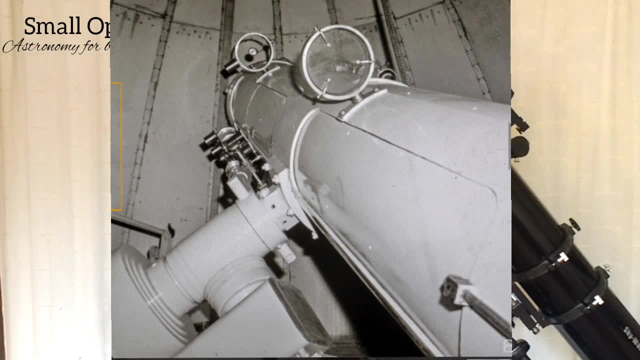 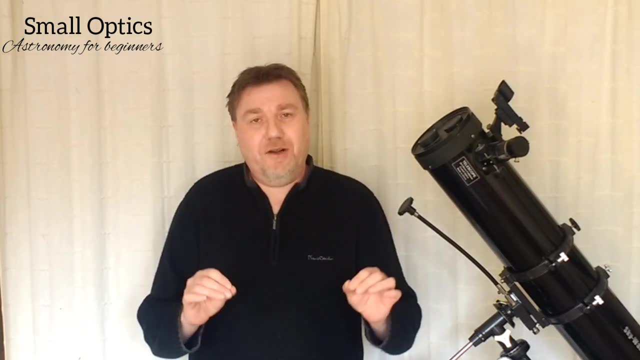 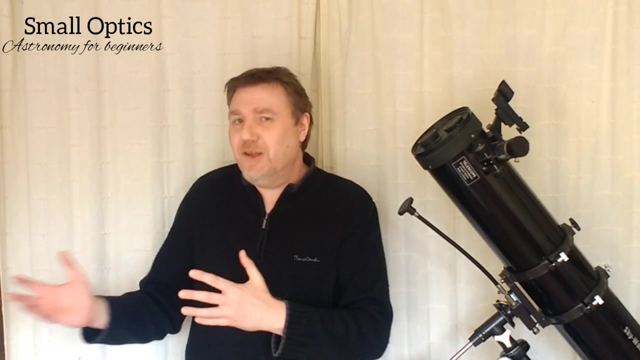 reflector and a lovely dome. it's a fantastic telescope and so, like I say, I was lucky enough to grow up with one of those. but the thing is with astronomy clubs or societies is: don't be worried about joining them because you know nothing about the night sky. okay, they'll accept people at all levels and, to be honest with you, they love beginners because there's nothing more an astronomer love is to share this amazing. 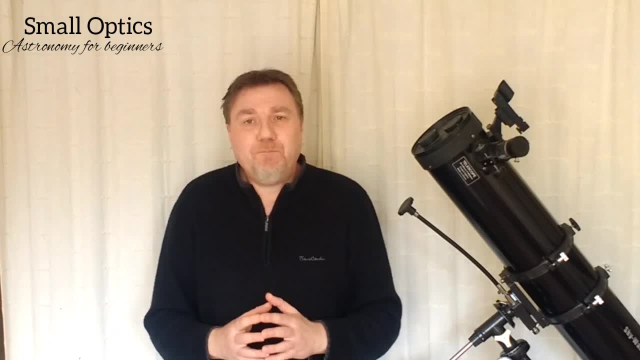 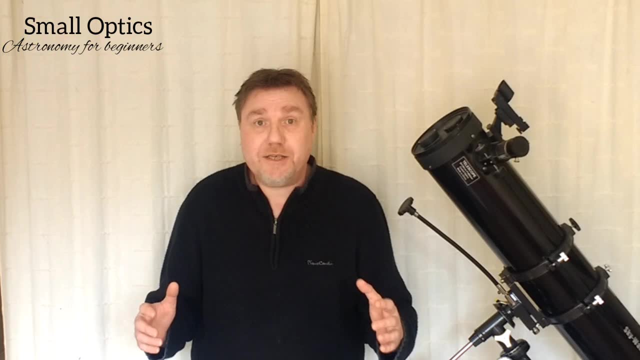 hobby, okay, and get you started. so just have a quick Google search and see if there is some kind of club that's nearby you. you may be surprised that there is actually, because there's quite a few dotted around all over the place and it's usually not that expensive. you don't need no qualifications or nothing, like you don't have to be some professor or something to join an Astronomical Society, and usually all they want to do is to get you started. 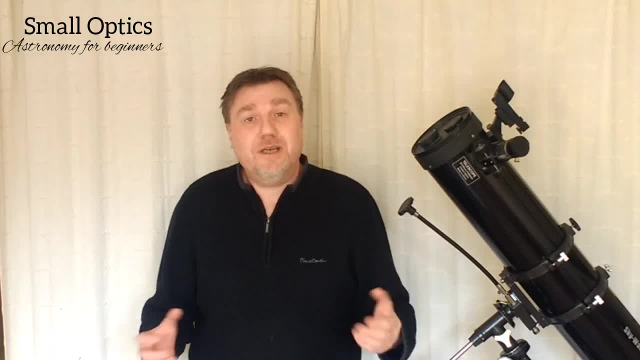 want the. well, I know this one at Chesterfield is just a small donation. usually, you know, throw a couple of pound in a bucket or something like that to keep the observatory going. but, like I say, it's full of really fantastic people where you're just going to be able to ask as many questions as you like. you're going to be able to use some amazing gear, some gear that you can only dream of. I know I have in my time up there and so you know I can't advise it anymore now if you haven't got a. 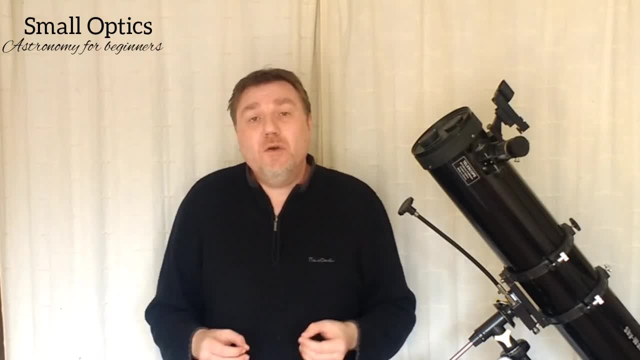 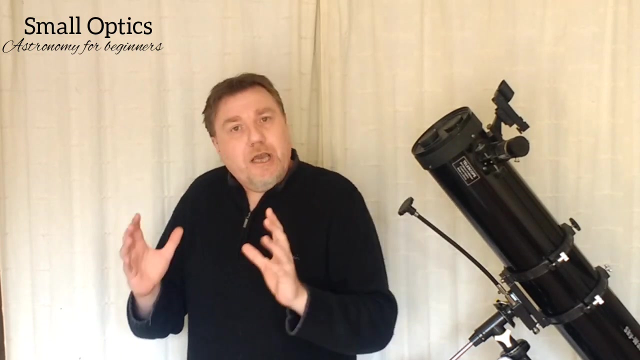 society nearby you. the next best thing would be some kind of astronomy group online group. now one of my subscribers has kindly set up a Facebook group for small optics. I'll leave a link in the description for that, and you're more than welcome to come in there, ask as many questions as you like, okay. so remember, it doesn't matter what level you are, just get yourself joined in some kind of group or society. you'll not regret it, trust me.